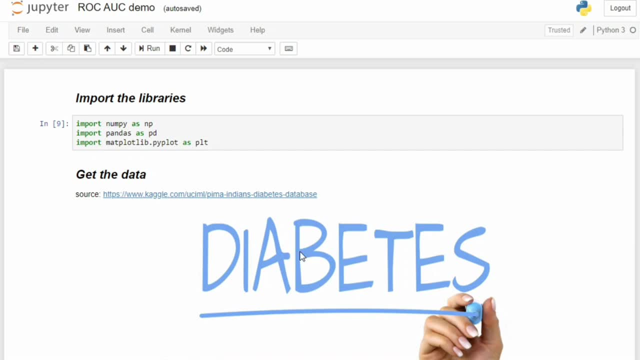 in patients. okay, So I have got the dataset from Kaggle and this is originally a UCI dataset and if you just visit this link you will get all the details that will be necessary for it and you can download the dataset. obviously, And to begin with, we are gonna import the famous trio: numpy, pandas and matplotlib. 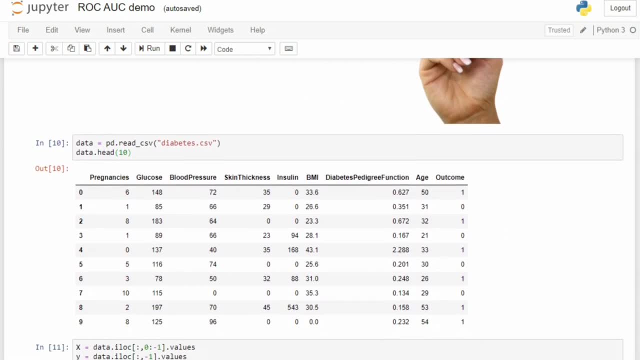 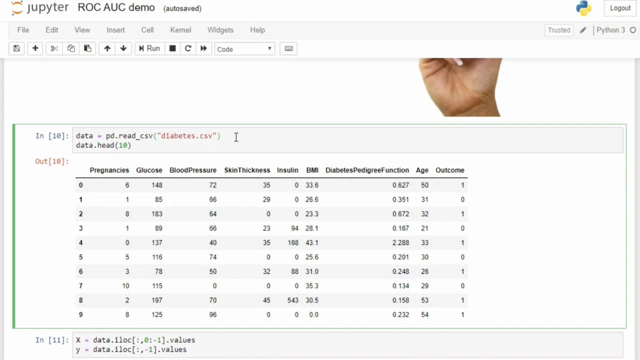 okay, So after doing that, we are obviously gonna read our dataset- and pandas is the best for reading the CSV dataset, in my opinion- and see that the parameter here I have passed is diabetescsv. So obviously this is my file name where this data is stored. okay, 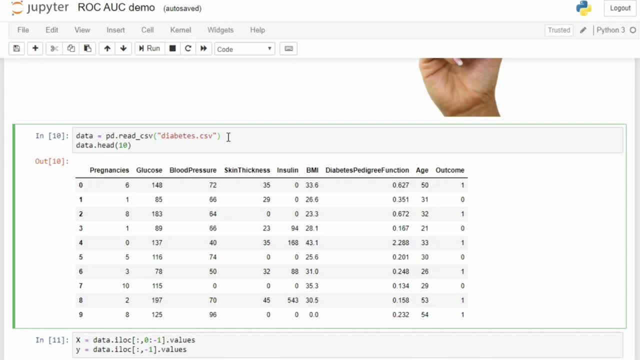 And as I have stored them at the same folder level as of my notebook, so I don't need to pass anything else in this path. After that, I am using the head function to show first 10 rows of our dataset. So let me quickly explain the columns to you, okay. 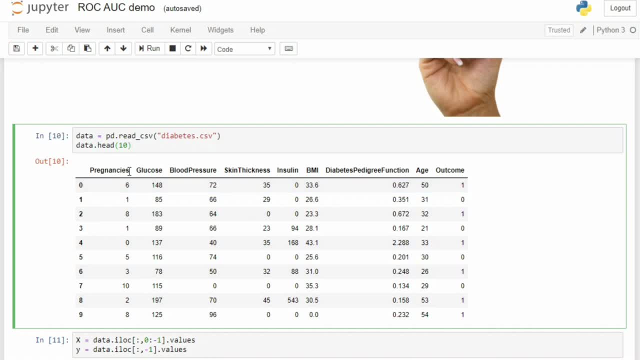 The first column is showing the number of pregnancies, So it simply means how many times the patient has gone through pregnancies. okay, Then we have the glucose, So this is showing the amount of glucose in the body. Then we have blood pressure, Then we have skin thickness. 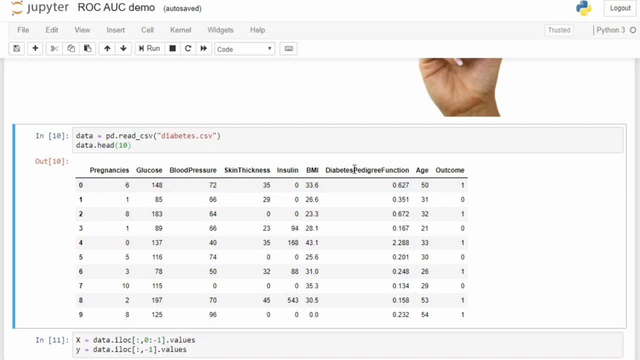 Then insulin amount, Then BMI, Then a function which is diabetes pedigree function here. I believe this is a kind of function which tells you the likelihood of having diabetes, okay, And then we have the age and outcome. Well, it is a binary classification problem. 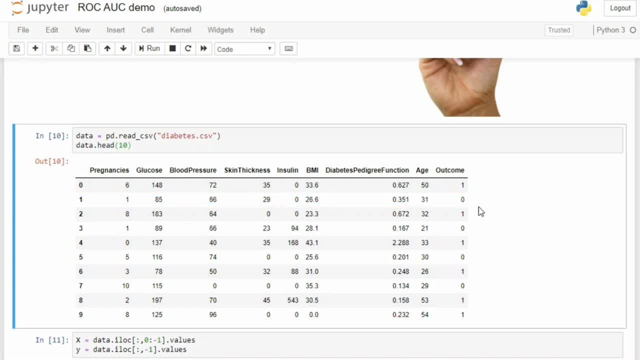 So we can have only possibly two outcomes: 1 and 0.. So 1 refers to the positive- Well, not from the patient side, Haha. So 1 refers to the fact the patient has diabetes and 0 refers to the fact the patient doesn't have diabetes. 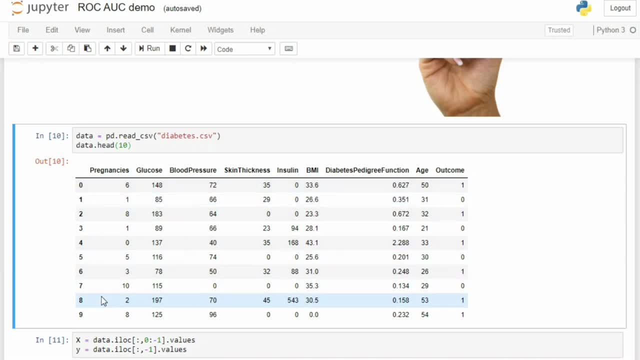 So ignore this column for a moment and focus on these columns. So these are the features, right, And you can see that there are many zeros and in this dataset, 0 denotes the missing value, the NAND values. okay, I am not gonna impute them because I am gonna be focusing on the ROC and AUC part. 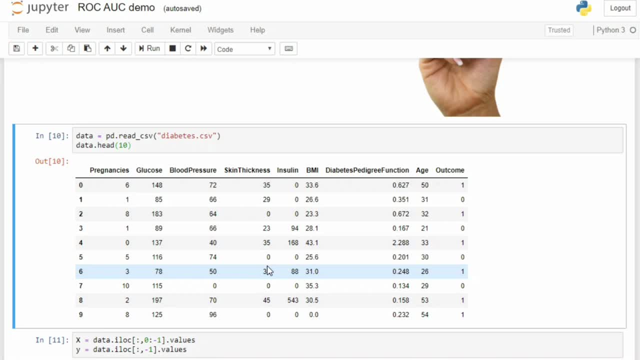 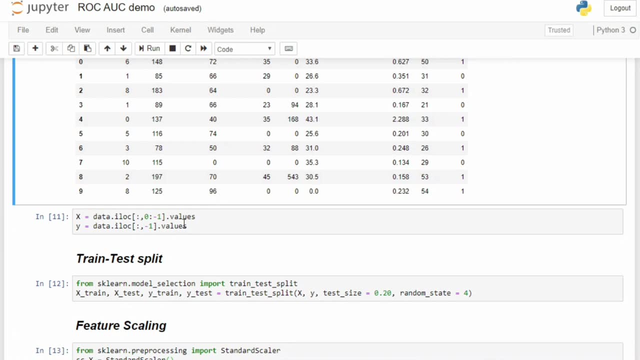 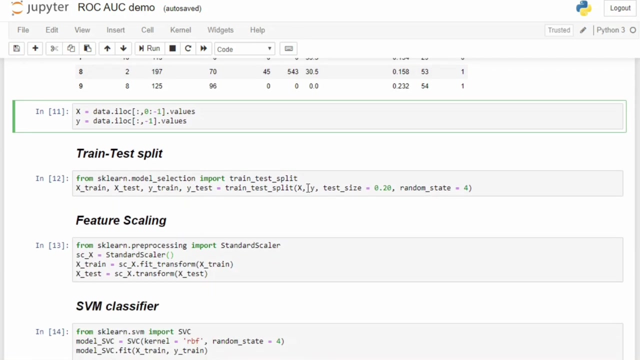 So really into this project. that is, if you really want to solve this problem, then you should probably impute them. so moving on. so this thing just separates our matrix of feature and the output vector. okay, now we have the train test split and you can see that I am using a test size of 0.2. that means 80% of my 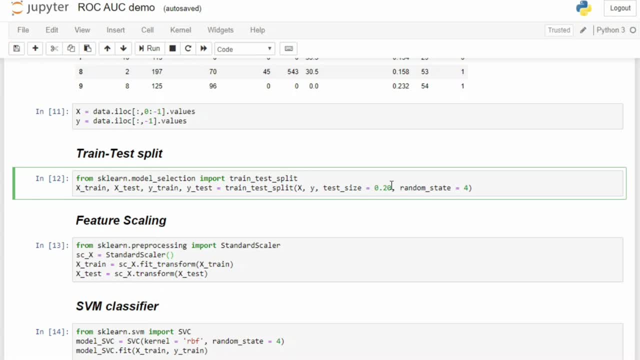 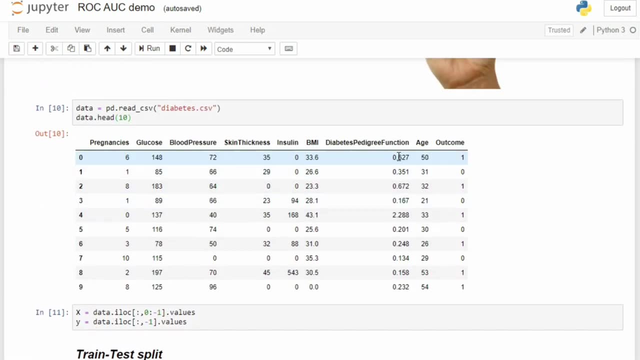 data will be used in training the model and 20% will be used in validating the model. now I have done some feature scaling here. as you can see, in this column the values are really low, but in other columns the values can get really huge. so it's better to do feature scaling in this case. okay, moving on to 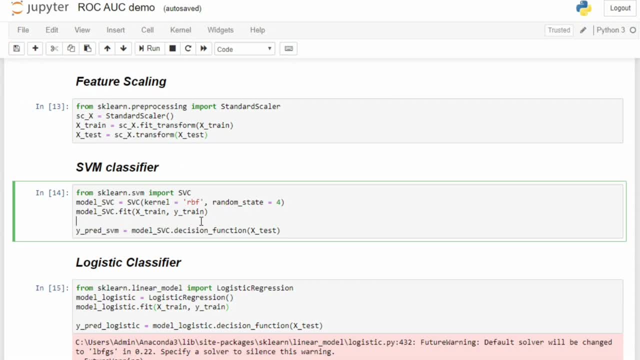 really show you how to use ROC and ADA. under ROC, I have actually built two models, okay, the first one is SVM classifier and the second one is logistic classifier. now you can see, I am using scikit-learn library to build our SVM classifier and I am importing the class SVC, which basically stands for support vector. 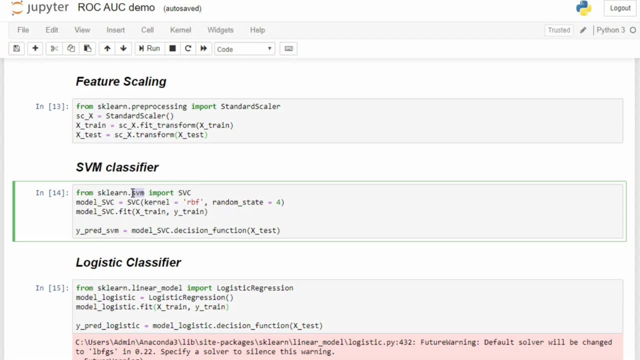 classifier from the module SVM of scikit-learn. okay, and here the kernel I am using is as RBF kernel and I am just simply creating an object of this class and I am just fitting the train data, that is, the X train and Y train, the 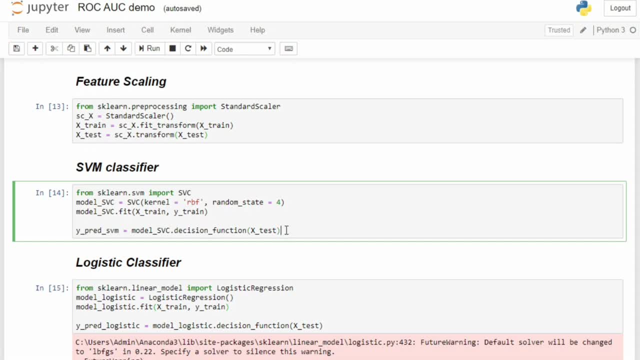 line I am just creating is the method of writing the train data. okay, and let's do that. okay. so what you're gonna do is: this is the function code that you can use. okay, so right now we are going to use RFC. I am using it because, like the 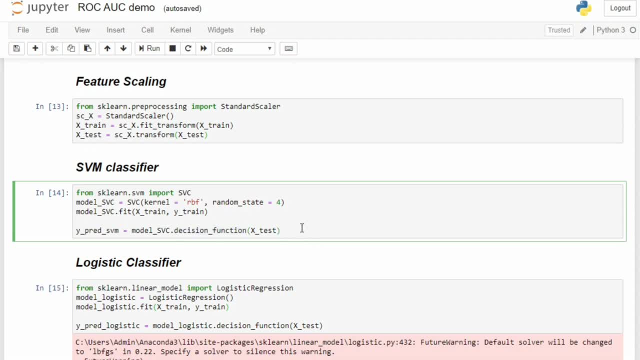 code. I am using it to predict the outcomes. okay, so let's say the task is to do a calculation of the number of actions. this is going to be the number function. okay, we are just going to create a function where we are going to do the operation of the number of actions, which is going to be the number of actions. 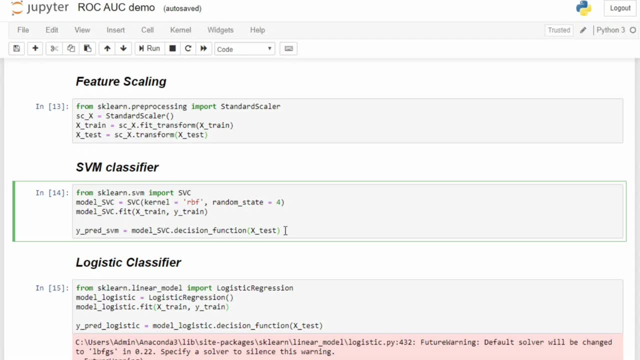 okay. so basically this is the function we are going to do- is we are going to do the n features? okay, assume that our classifier is just a plane in that nth dimension. okay, so what this function will actually return is the distance of this point from that plane. but when we 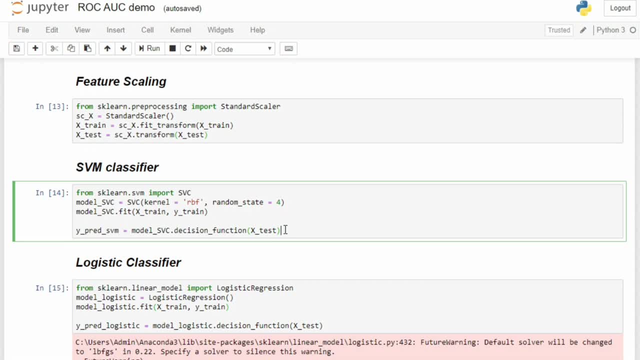 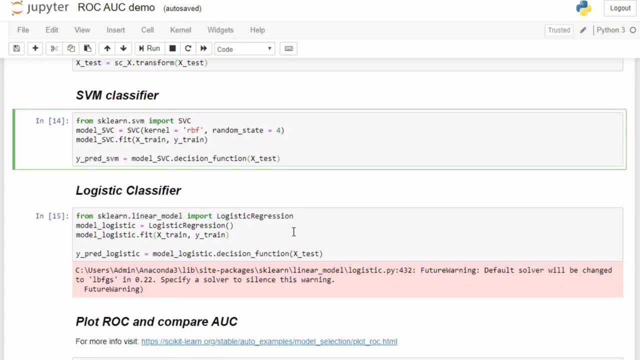 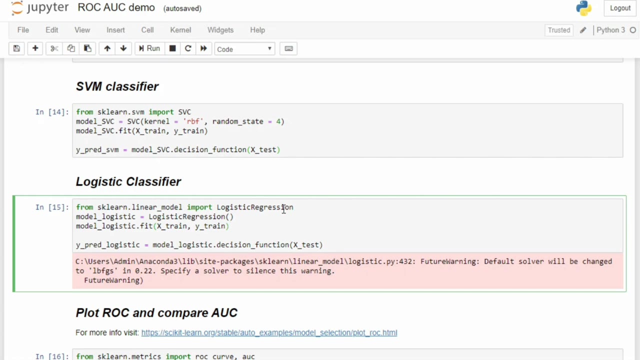 use a predict function that will give us a probability value from 0 to 1, but this function can give you even negative values. okay, so, moving on this logistic classifier. well, again, i am using the cyclic library to build our logistic classifier and the class we need to import. 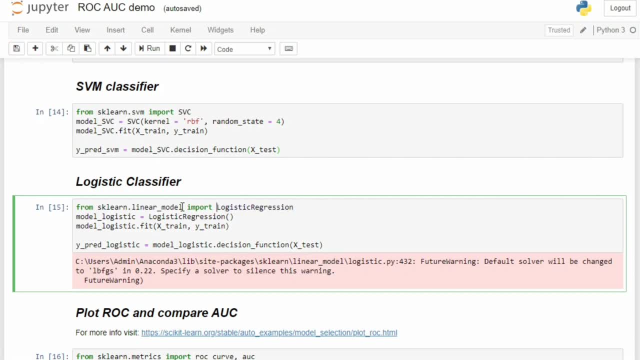 here is logistic regression from the module called linear model of a skill and library. now again, i am defining an object of this class, then i am fitting it on my training data and again i am computing. the decision function okay. so so far we have built two models and 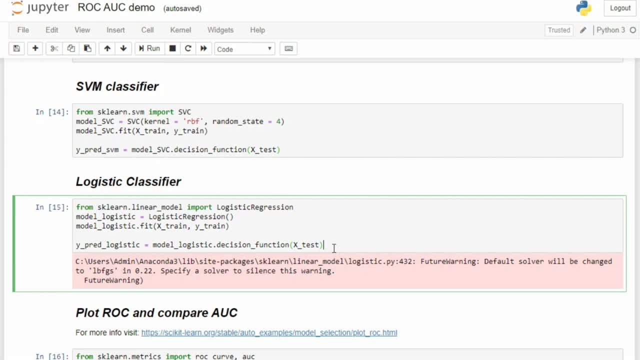 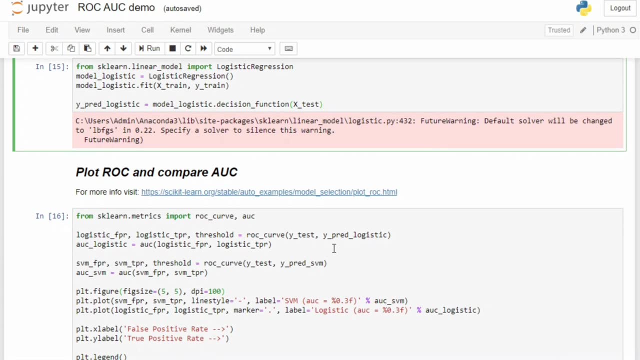 calculated the decision function of our logistic classifier and i am computing the model of this model. and i am computing the decision function of our logistic classifier and i am computing the decision functions. okay, now we are gonna plot them, so i would like to remind you quickly what is. 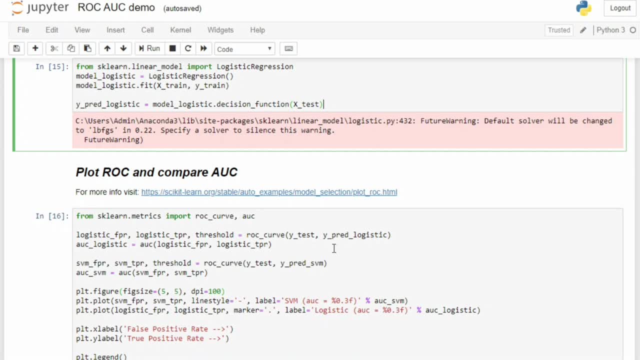 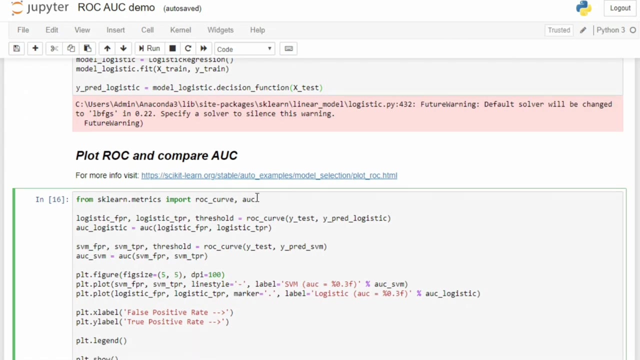 roc plot. basically, it is a plot between true positive rate and false positive rate. in the y-axis we have true positive rate and in the x-axis we have false positive rates. okay, so we need to calculate them, and scikit-learn actually offers two classes here: roc, curve and auc. now, obviously, 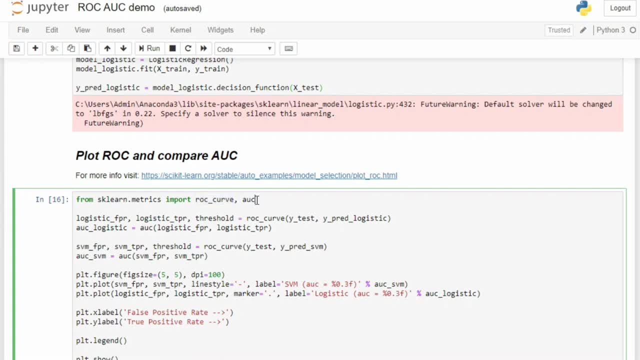 this we will be using to plot the graph and this we will be using to compute the area under the roc curve. okay, now we need to determine what are the true positive rate, false positive rate. okay, so actually this function returns three things. first one is false positive rate. second one is: 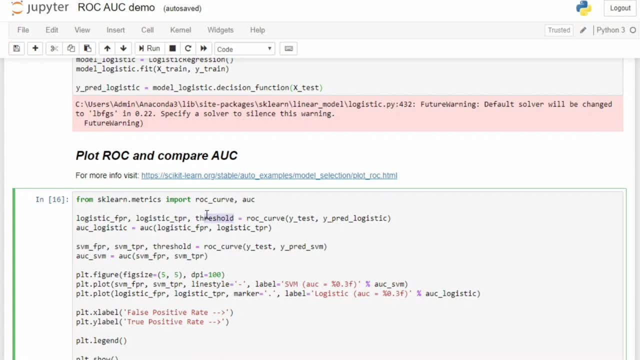 true positive rate. and the third one is threshold. well, we actually don't need threshold here here, but if you want to know what is the threshold of a point in the graph, you can use this one. that's why i have written it, so you can see that i am first computing all these things for logistic. 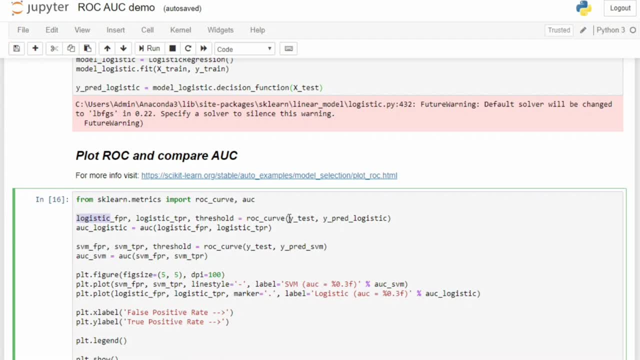 hence this prefix logistic. and this function actually takes two arguments. the first one should be the ground truth, that is, the y test, and the second one should be the decision functions. okay, and here you can see the ad end of the curve can be easily found by this auc function. 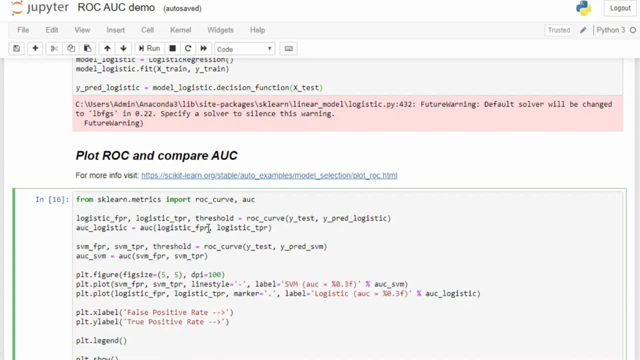 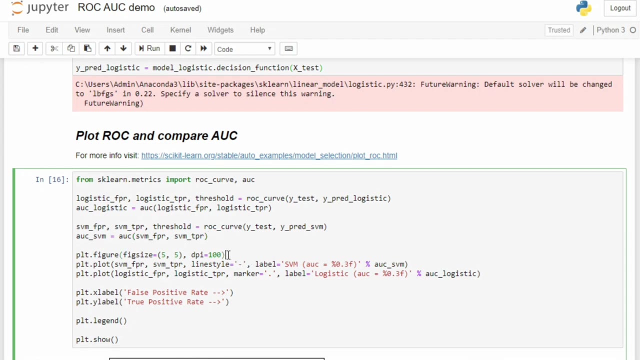 and it just takes two values: the false positive rates and the true positive rates. okay, so similarly i have done the thing for svm classifier also. now comes the interesting part. we are gonna plot it now. obviously i'm gonna use the matplotlib library for that. so figure size: i am taking it as 5.5 and the density of pixel per inch is 100. 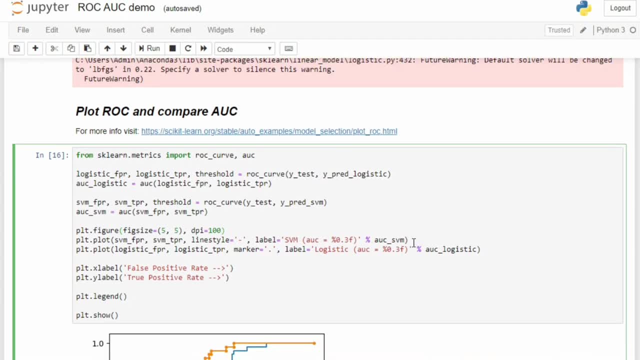 so now i'm gonna plot it well. you can just copy and paste this code- this is really simple one- and some little decoration here: the false positive rate and true positive rate levels. then i have also included the legends and, lastly, the show. okay, so after running this, you will get something like this: okay now. 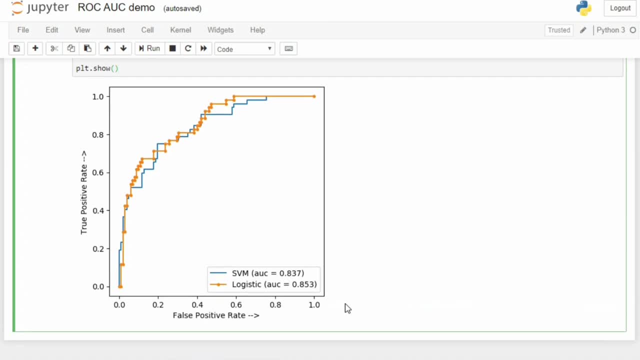 comes the really interesting part, because now we are going to analyze it. so by this legend we are told that the orange line- i guess it's orange orange- the orange line denotes logistic curve and the blue line denotes the svm curve, and you can see the ad under the curve. 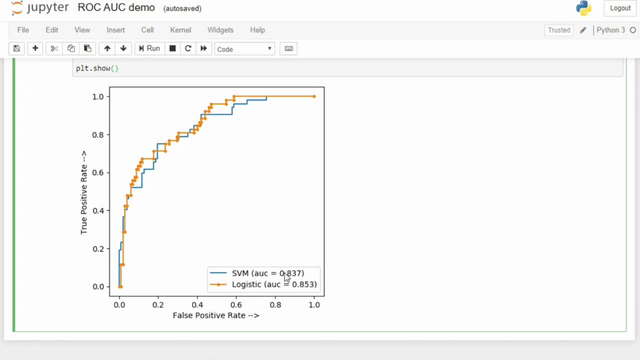 for logistic is greater than the area under the curve svm. so if you have watched my previous video, then you know that a larger area means a better model. so what would you choose in this case? well, obviously, we would choose the logistic regression in this case. all right now. 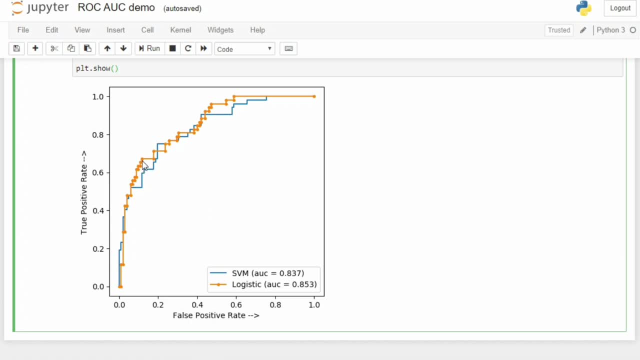 look at this point. okay, so you can see that at this point the true positive rate is really high and the false positive rate is really low. now, if we just draw a vertical line, imagine a vertical line here. okay, so you can see that for the same false positive rate, 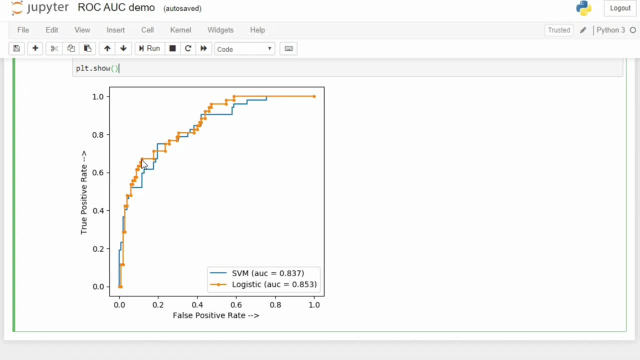 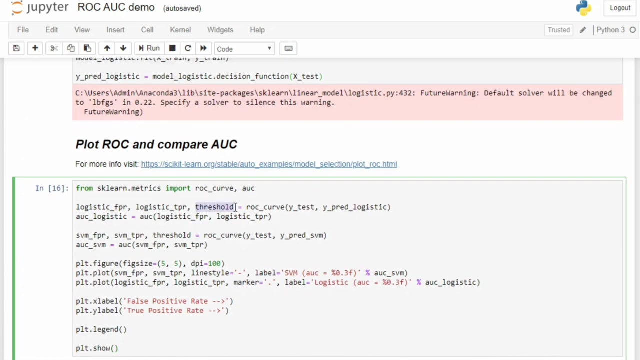 at this point the true positive rate is higher in case of logistic curve and lower in case of svm curve. so that actually tells you that, okay, if our aim is to maximize true positive, then we should probably go for the logistic curve and at this point and the threshold value you can find by this array, okay,